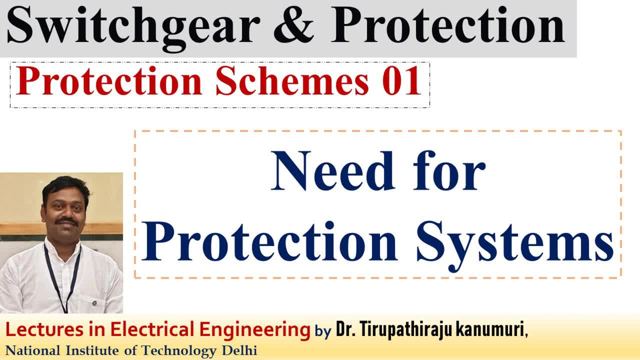 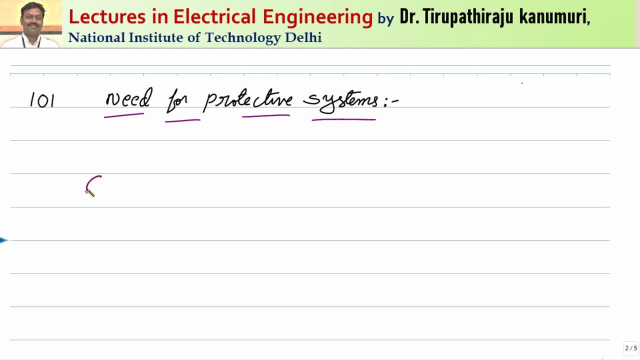 Hi all. today we are going to discuss about need for protective systems. What is the need for protective systems? Why should we go for the protection? So if you are taking your power system, I am just drawing the single line diagram for the power system Having a single alternator. 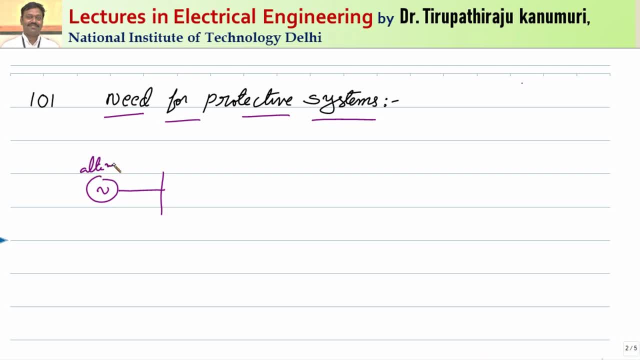 so the, basically it will contain an alternator. So the alternator will be connected to a bus bar, then followed by a step-up transformer, Then the high voltage transmission is done and in between some switching substations may be there and there it may be divided into further. 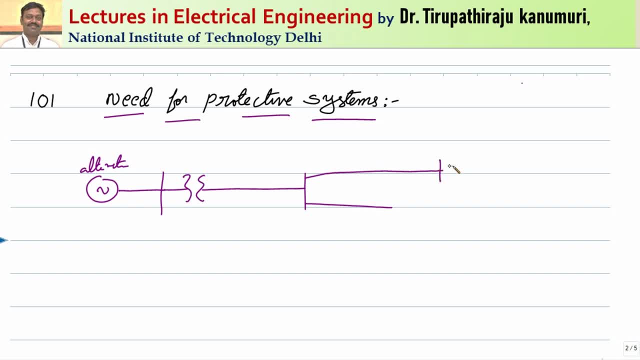 into parts. Let us assume again, this is again connected to some transformer. So let us take, for example, this is connected to some transformer and from this it is again subdivided into some small parts. So it is subdivided into small parts. This also subdivided into small parts. 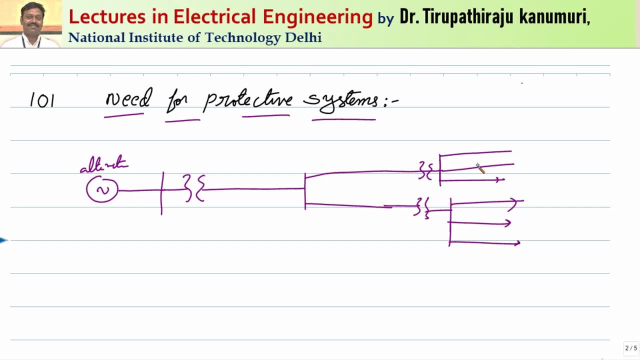 like primary transmission, secondary transmission, different type of transmissions are there. Let us take for example here. some load is there, So this load can be either normal normal load or this load can be even motor also. That means it will have different parameters. 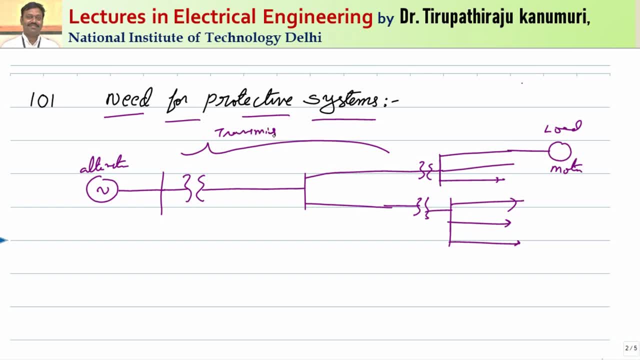 They are the transmission line and similarly there will be a distribution line. These are the basic components, and there are transformers, There is alternator, as well as there can be some motors also either. That means the current phase of the load has been determined, So the load has been determined. 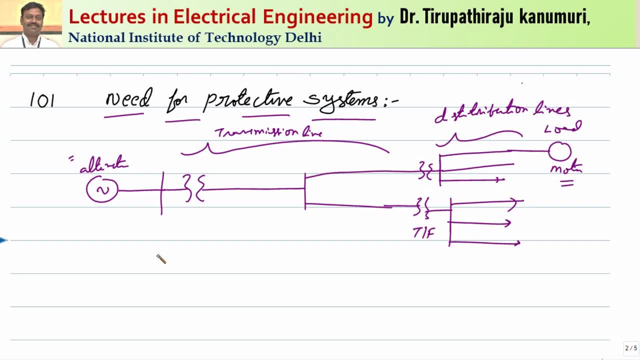 Then there are also the synchronous motors or the induction motors, which will cause the problems, which are the main, big, big components in your power systems. And along with this, nowadays we are going for the interconnected power systems, Where, in the interconnected power systems, the alternators at different points or the generators at or the power stations of different locations are interconnected to maintain the continuity of supply. But basically the components that will be existing will be these things: only: The alternator or a generator. the transformer will be there, the transformer will not be there, So the power station will be there, the. 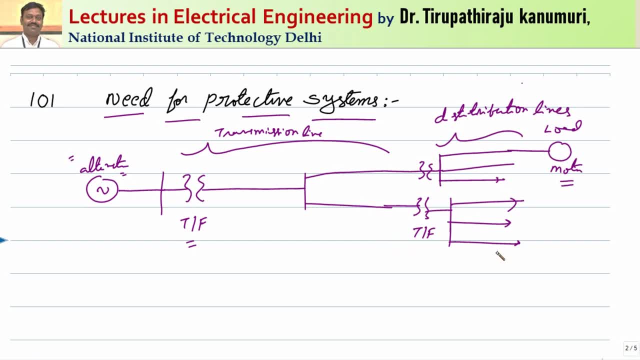 voltage will be there, as well, as the inner power station will also be there. The ground transmission lines will be there and distribution lines will be there, and here we can go for either overhead transmission lines or underground cables and at the load, the major things that 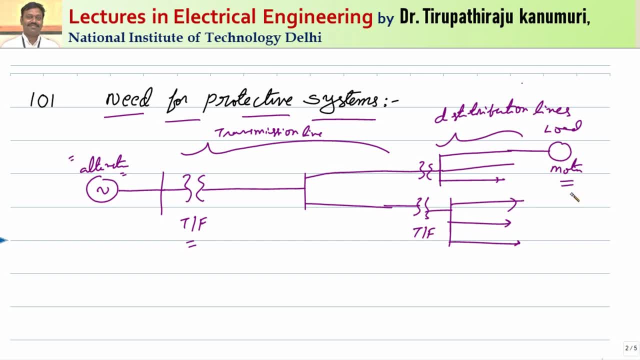 are going to affect are the motors, because remaining things are not going to contribute for the fault whenever the fault comes. So now let us see what is the meaning of the fault. What is the meaning of the fault? The fault is nothing but any defect in any part of the system. 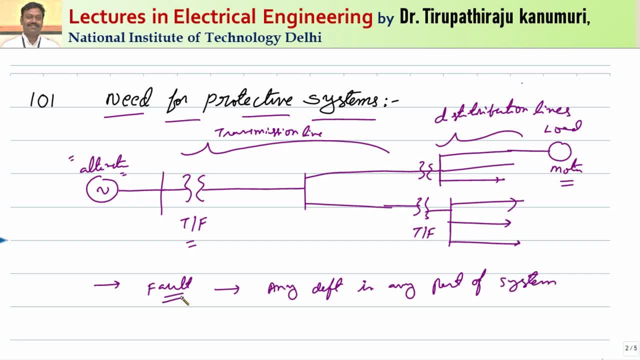 So if there is some defect in any part of the system that we name by the term fault, So fault doesn't mean it is a short circuit, please remember. So the fault can be either open circuit, So which happens to the breakage of the conductors, or it can be the short circuit. 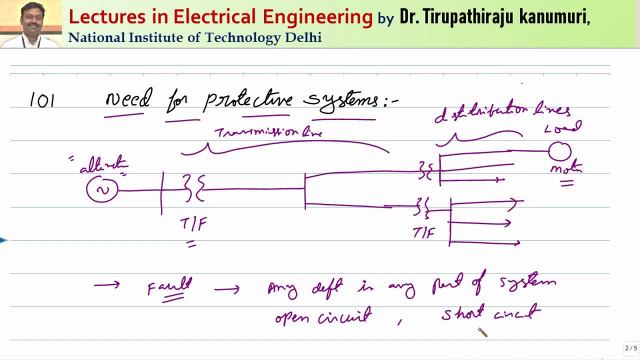 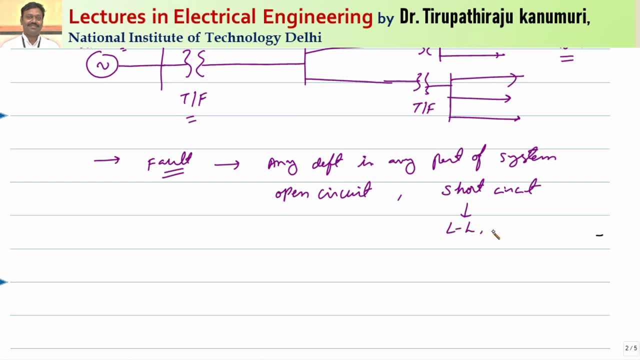 So the short circuit. again, this can be divided into different types. The short circuit can happen between two conductors, that is called as a line to line. or it can happen between one conductor to ground, that we can call as LG. or it can happen between two conductors and then to ground, or it can happen between the three conductors or three. 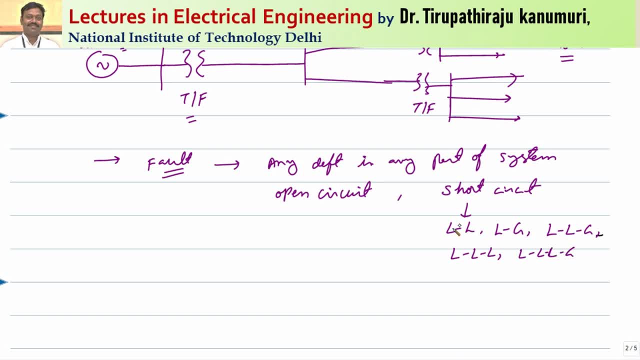 conductors to ground So any type of fault can be there. That means two live conductors are connected together or any live conductor is connected to ground In all these cases because the current increases drastically. in the case of short circuit, the current increases, the voltage falls down. 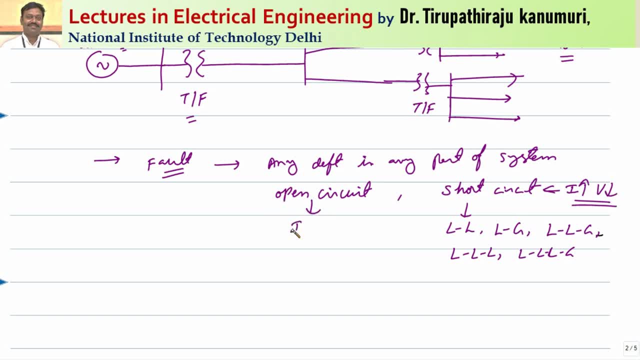 This is the property of the short circuit. In the case of open circuit, the current becomes zero and the voltage increases as a result of this, because we know our power system or a transmission line consists of the energy storage elements. They are the inductor and the capacitor, because they doesn't allow the sudden change in the 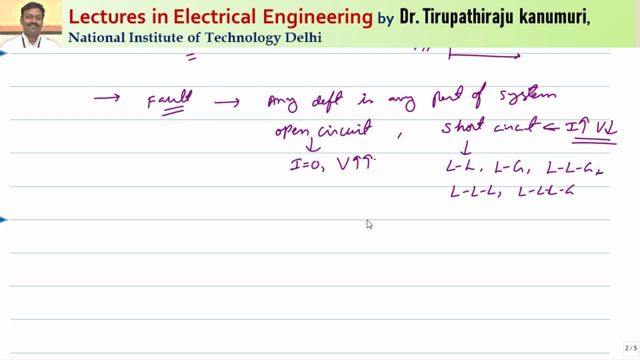 characteristics because, as that doesn't allow the sudden change in characteristics, Whenever you do the open circuit, the inductor will try to transfer its energy to the capacitor because the current is becoming zero, So automatically voltage will rise, Whereas whenever the short circuit happens, the capacitor will try to transfer its energy. 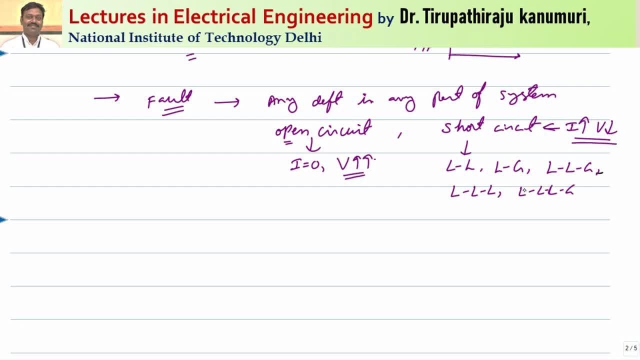 to the inductor So the currents increases drastically. So these things we have studied in transmission lines, in the traveling waves. If you have doubt you can please refer there. There I have discussed all these things. whenever the switch is closed or short circuit happens, 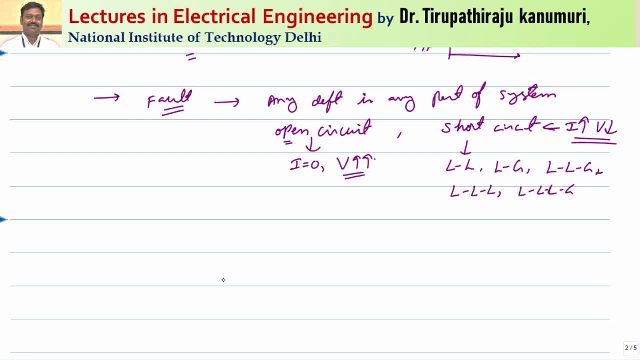 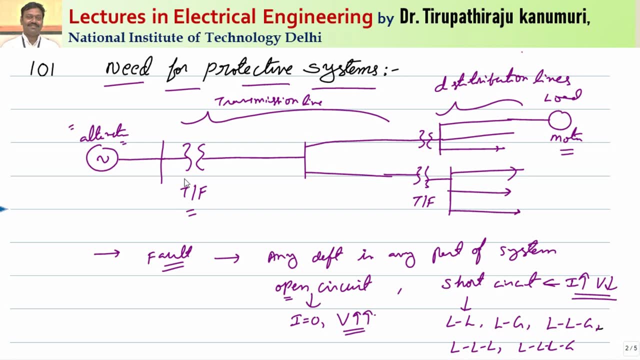 how the circuit behaves Under transient conditions. So now this fault can happen on any one of these systems. Let us briefly discuss about different types of faults that can happen. So if you are taking the transmission line, for example, so the transmission line, the 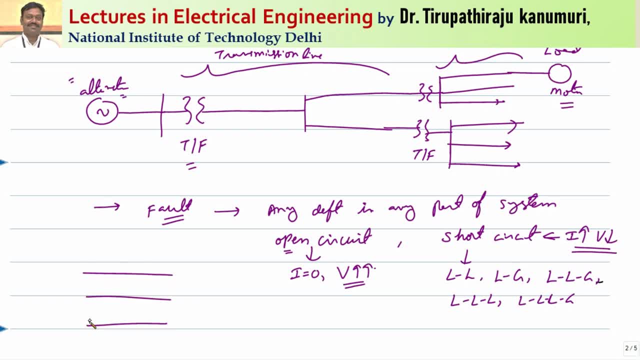 faults can be because transmission line basically consists of three conductors and each conductor will have the insulation Either this overhead transmission line. for example, they are connected to an insulator. Through the insulator they are connected to a cross arm, So the fault can happen between this conductor. 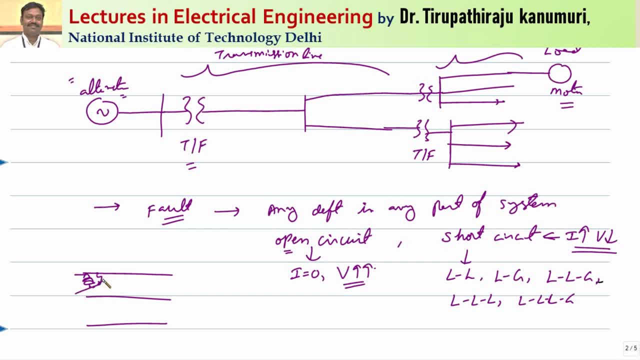 And this cross arm, because cross arm with the ground potential, here the short circuit can happen or flash over can happen. because these flash overs can happen because of switching transients or lightening strokes, Because during switching transients or lightening strokes the voltages increases drastically. 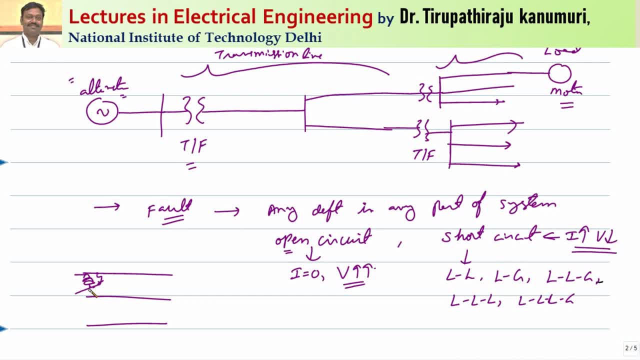 Why they increase. We have seen in the traveling waves in power systems. You can please refer there. Similarly, some bird or some animal or something can come, some object like, for example, during wind or rainy season, Some plant may come and fall on the transmission. 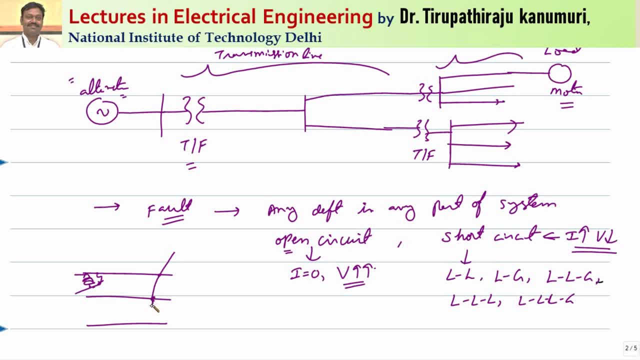 So this is the short circuit, This is the transmission line, So the plant can fall between two conductors or it may touch all the three conductors. So this will be accordingly, it will be converted to the equivalent fault. or sometimes the bird sitting on any one conductor while flying from there may short circuit two adjacent 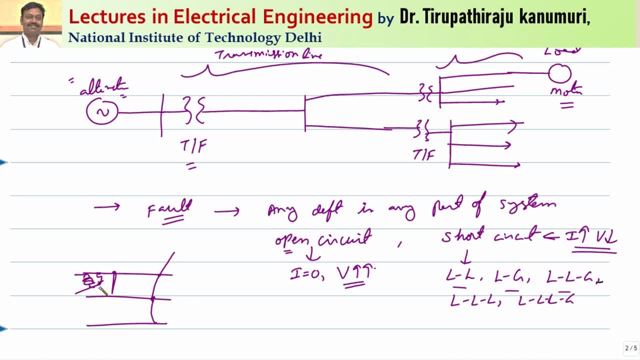 conductors or may do the short circuit between conductor and the cross arm. So in that case also the fault can happen And similarly some other type of faults that can happen is because the insulators are there. with respect to the time the moisture will get absorbed by these insulators, 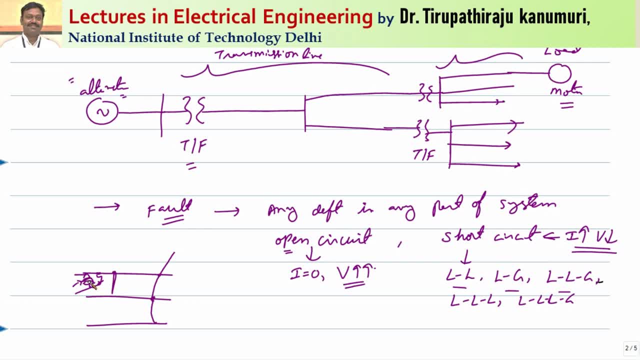 Like, for example, if it is near to the cement industry, the dust get accumulated, or if it is near to the seashore, the salt will get condensed on these. Because of this, there will be continuous leakage currents and sometimes during the switching, transients or surges. 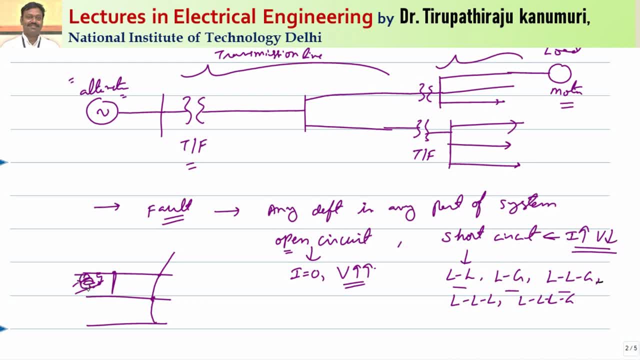 So the flashover will happen between the conductor and the cross arm. So this is also one more reason that can happen in the case of transmission lines. And one more case that can happen is in the transmission line we do the joint of the conductors in between. 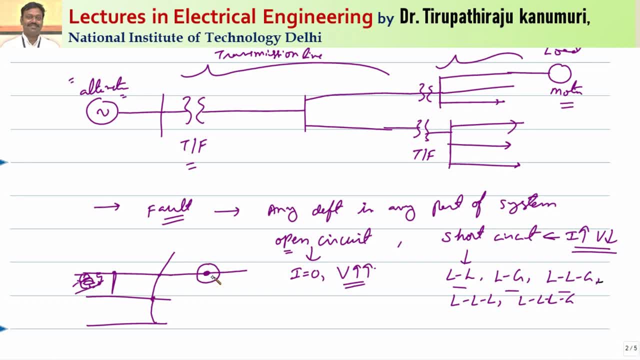 Sometimes The joint will break when the joints are broken. So if it is in between the line- that means between two towers- the conductor will fall on the ground. So this leads to the ground fault or short circuit fault. If this joint is near to the tower, or by opening the joint, let us assume no conductor has. 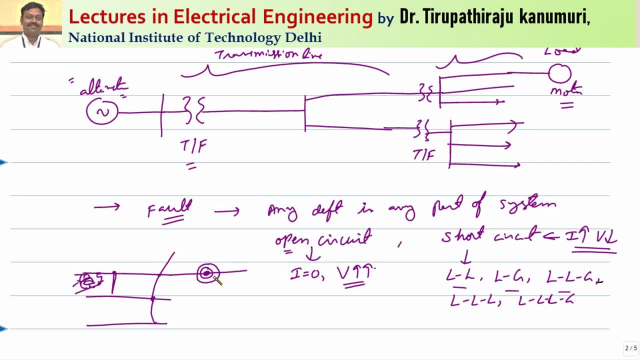 fallen on ground, then it leads to a open circuit fault. Similar is the case for the cables, also because the insulators may fail, that may lead to the problems. Now coming to the alternators, transformers or motors, Because there two adjacent conductors are protected by the insulation. 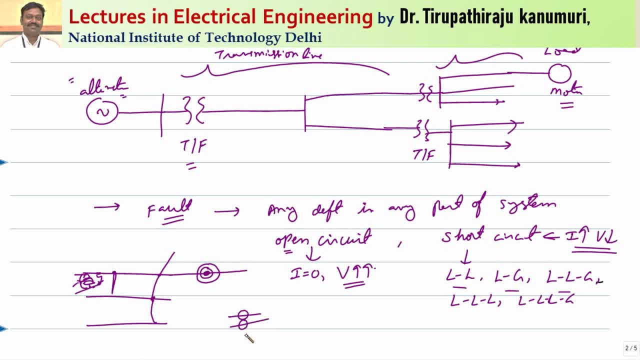 That means if you are taking two adjacent conductors, they are protected by the insulation. So with respect to the time, we have seen again in the power systems, in the cables that with respect to the time the cable absorbs the moisture. So same thing is the case for the conductor where the insulation is there. 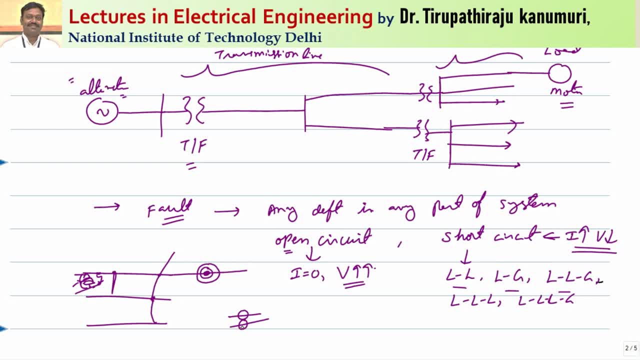 With respect to the time the insulation absorbs the moisture. Because of absorbing the moisture, it loses its dielectric strength and because of that the leakage current may start passing from them, And sometimes the breakdown may happen between two conductors that may lead to the faults. 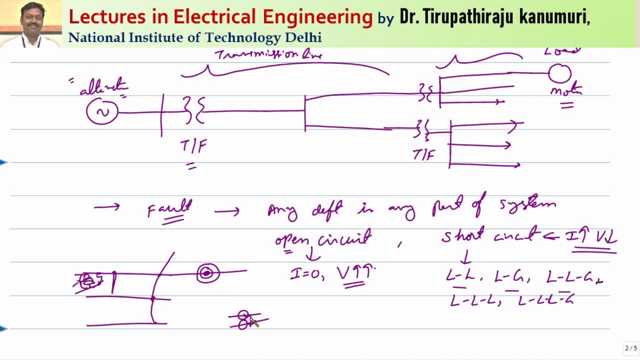 That means if you take the transformer or the alternators. these faults are called as inter-turn faults or inter-phase faults, because this can happen two adjacent phases or between two adjacent turns. Accordingly, they are called as inter-turn faults or between-phase faults. 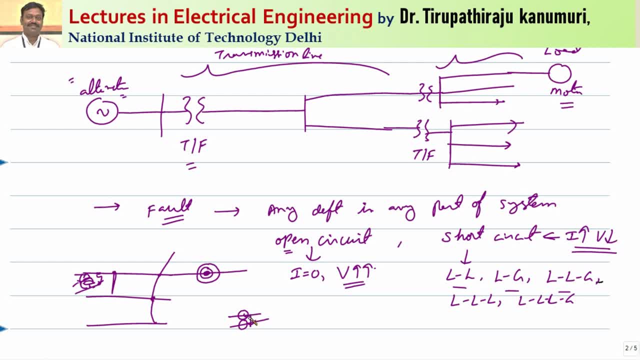 Similarly, in the case of cables, it can be caused between two adjacent phases. So generally, if this type of faults happens in the case of generators, transformers or cables, This is called as permanent faults, Whereas the faults that happen in the power systems may be transient or intermittent faults. 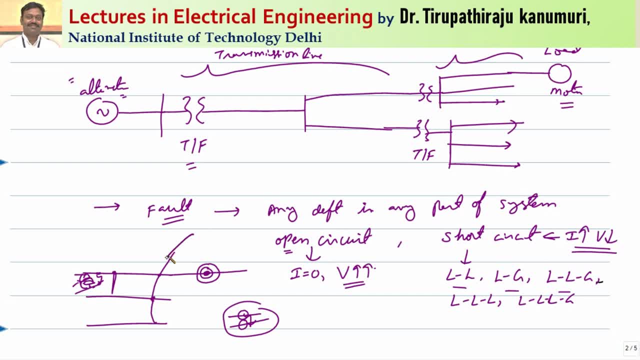 or permanent faults. That means the fault can happen because a plant come and fall on this branch of the plant. So whenever the plant branch falls on, this short circuit happens, So so much heat is produced there, because the spark will come there, So because of this the plant branch will burn and after some time this fault may disconnect. 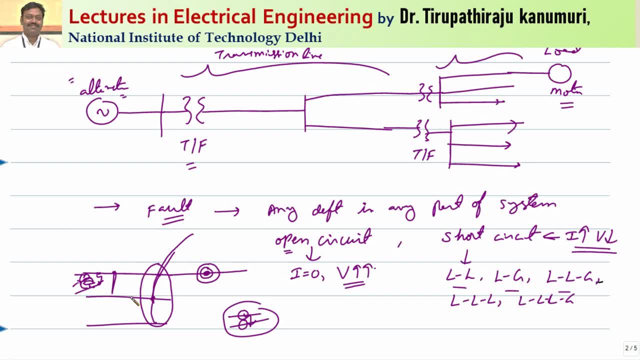 Similar is the case the bird. the bird, if it is touching two adjacent conductors, immediately the bird will die or fall Or fly away from there, So immediately that fault will get disconnected. So these cases are called as intermittent faults. And if the fault is permanent, like the conductor has broken, fallen on the ground, then it 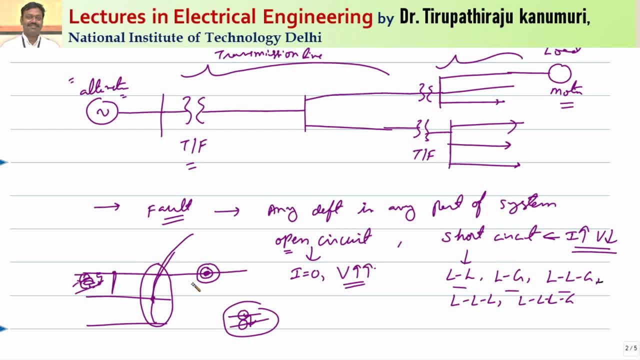 leads to the permanent faults. So in case of transmission line they can be intermittent faults or the permanent faults. So that's why, generally, recloser of your circuit breaker is done in order to check whether the fault is a permanent fault or a temporary fault, whereas that type of thing is not done. 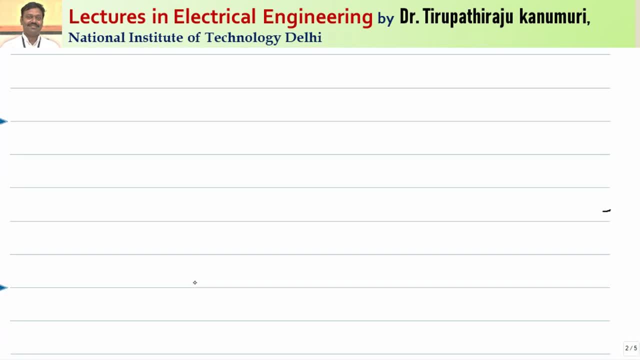 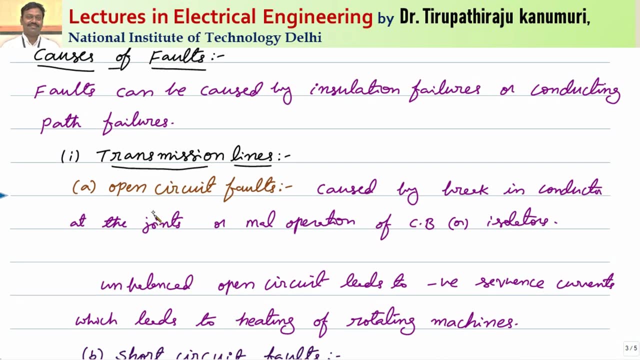 in the case of cables or alternators. I hope the basic things are clear to you, So now let us try to analyze the things one by one. So now I am discussing starting with the causes of the faults. So the faults can be caused either by the insulation failure or conducting path failure. 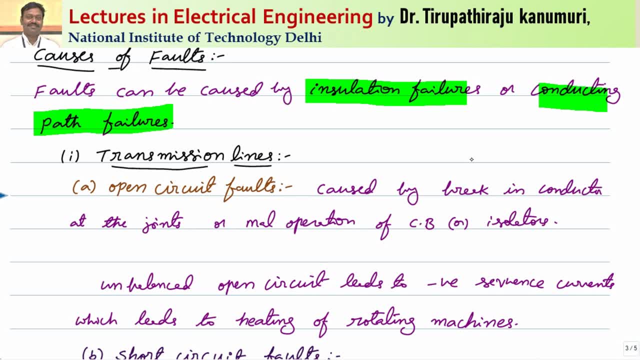 Conducting path failure means failure of the conductor. The conductor is broken. Insulation failure means the conductor is touching either to the ground or touching some another phase. So now, if you are taking the transmission line, the transmission line can have two things. 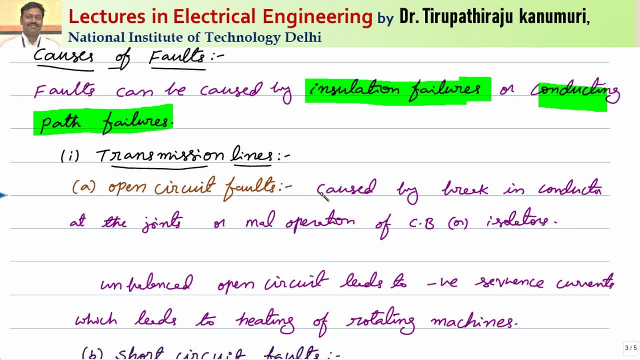 either open or closed, The open circuit fault or the short circuit fault. Now coming to the open circuit fault, the open circuit faults are caused by break in conductor at the joints or mal operation of circuit breaker or isolators. and coming to the unbalanced or open circuit faults, 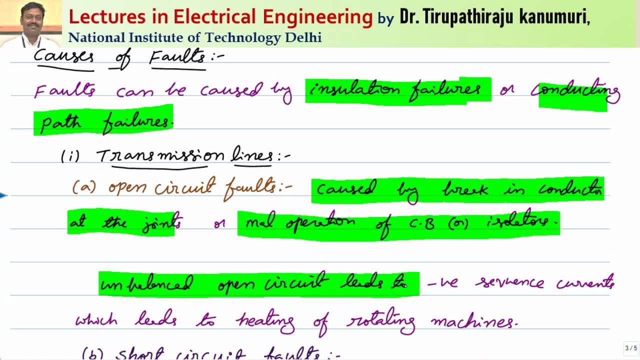 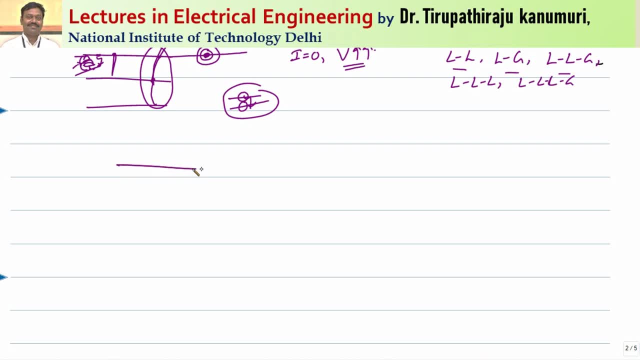 So this open circuit faults whenever the because let us assume I am having a three phase system. So I am again going back to this. Let us assume I am having three phase system. that means three adjacent conductors are there And between. let us assume there is some circuit breaker in between. 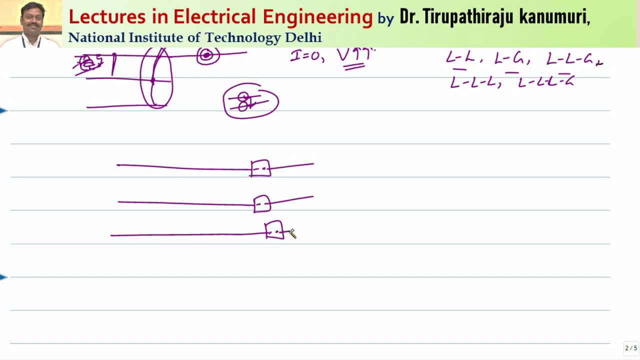 So circuit breaker is there or some isolator is there, So some switch. So during some operation, let us assume two circuit breakers have closed and this one circuit breaker has not closed the contact. Now what happens? Current will pass in these two. 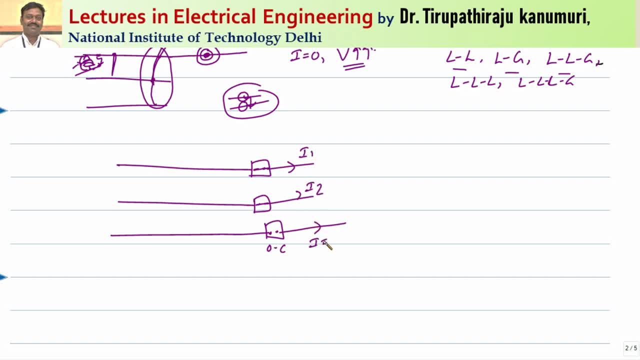 Current. I1 will pass here, I2 will pass here, but here the current becomes equal to zero. Because of this, what happens? Imbalance comes in the current. So whenever the unbalanced current comes because of open circuit, That means only some of the current comes. 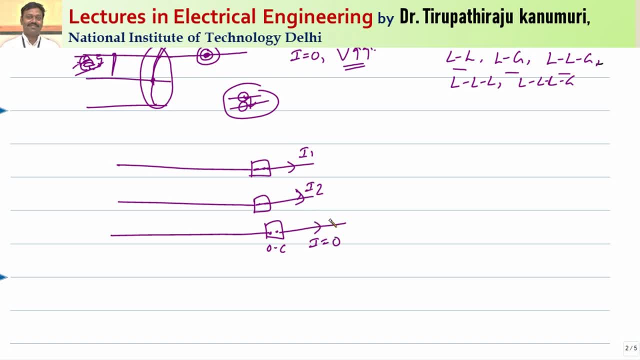 Only some phases are open circuited, not all phases. So this leads to unbalanced currents. So we have discussed in the power systems This unbalanced circuit or the unbalanced load, even the same thing I have discussed in the case of the basic electrical engineering, also unbalanced loading of a three phase. 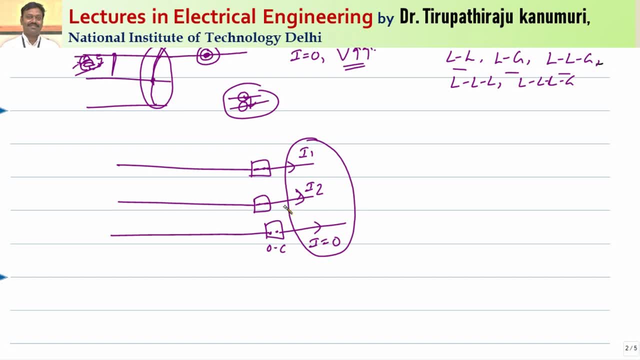 circuit. Wherever the unbalanced loading is done in a three phase circuit and if the three phase circuit is star connected, so this leads to the circulation of negative sequence currents. That means The unbalanced system can be represented as the sum of positive, negative, one zero sequence components. 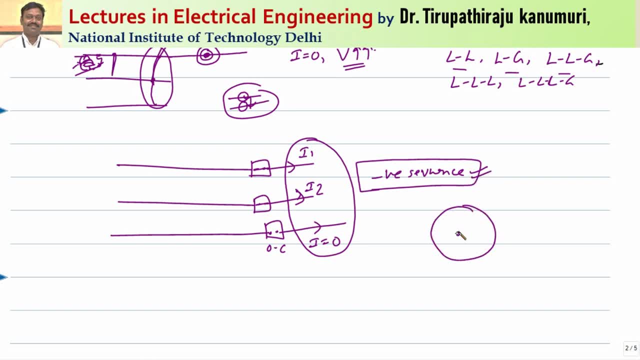 And the negative sequence components will start passing. Now, if you're taking a motor or generator, Let's assume the positive sequence components are rotating in this direction at a speed of NS. this negative sequence components will rotate in the opposite direction with the speed of NS. 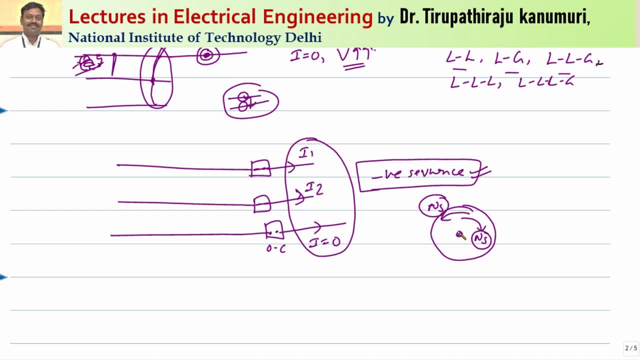 Or the relative speed between the positive and negative sequence components will be two times the speed, relative speed between the stator and the rotor. So because the speed becomes now two times of ns, because relative speed is with respect to the rotor point, this will be ns and ns two times of. 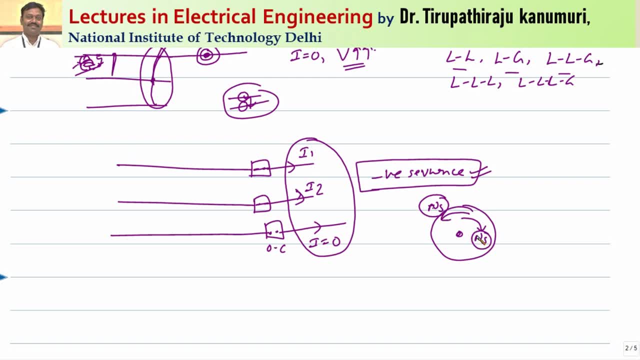 ns, So huge value of the voltages are produced. that leads to huge value of the circulating currents and lead to damage of your rotor. So these things I am going to discuss in the fault analysis, also in detail, where we discuss about the sequence components there I will discuss these. 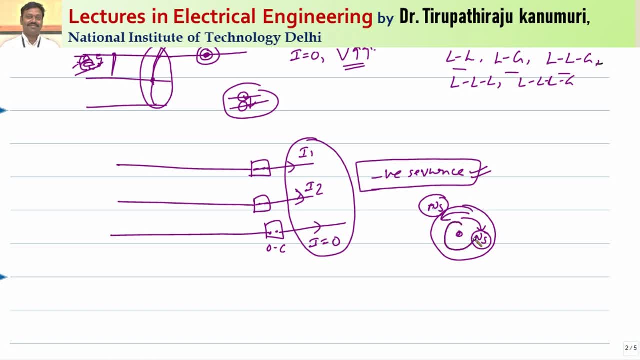 things in detail and I have discussed the same things in the harmonics of the machines also. you can please refer there if you have the doubts. I have discussed this in the damper winding concept. So in the damper winding I have discussed how the negative sequence components will lead to. 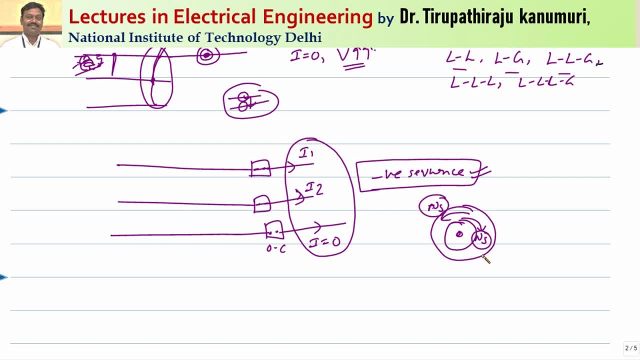 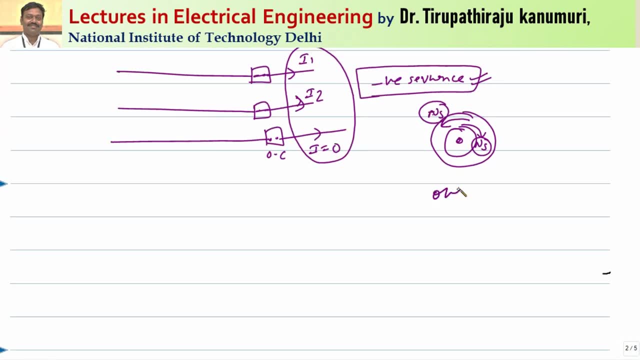 increase in the value of the voltage, So getting it so this leads to complete imbalance in the system. or because of this current, so much overheating of your machine happens, So because of this, this leads to overheating of your machines. So similar is the case for the faults. 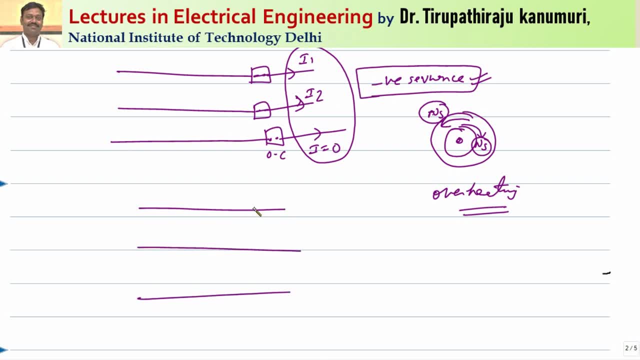 So the faults? if you are taking three conductors, so this fault can happen between a conductor to ground. So let us take assume this is connected to ground. this is called as a line to ground fault. Line to line fault means two adjacent conductors are connected together. This is called as a line. 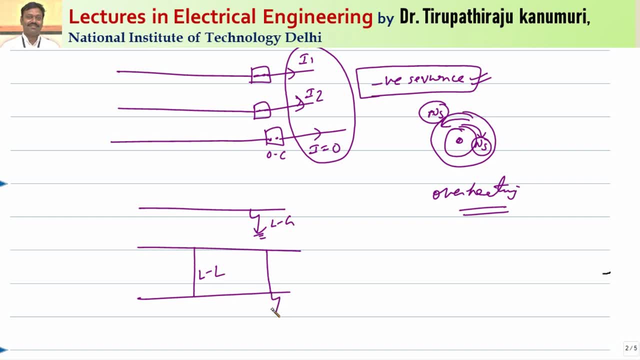 to line fault If two adjacent conductors are connected together and connected to ground. so this is called as a line to line to ground fault. and triple line fault means all the three phases are short circuited, So this is called as a triple line fault. and if it is connected to ground. 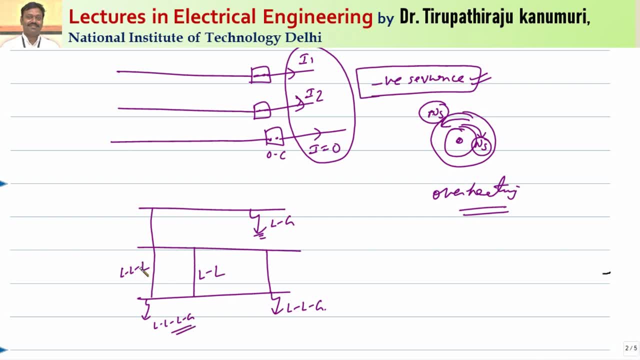 so then it is called as triple line to ground fault. So, out of these faults, triple line faults and triple line to ground faults, because all the three phases are affected equally- the condition will be the balanced current, even though the current magnitude is more, but it will be balanced. 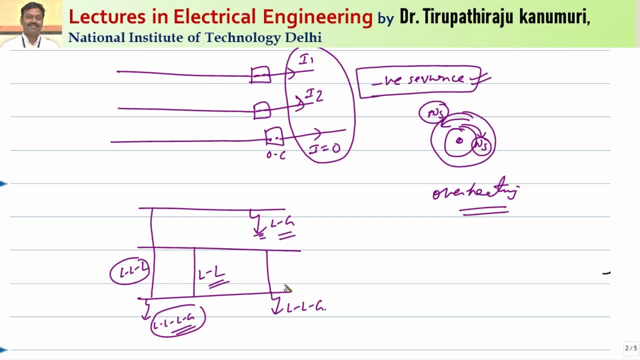 whereas if you go for the line to line fault, line to ground fault or double line to ground fault, in that case the currents will be different in the different phases, So this will also lead to same type of effect in the machines. So these are the problems with these faults. 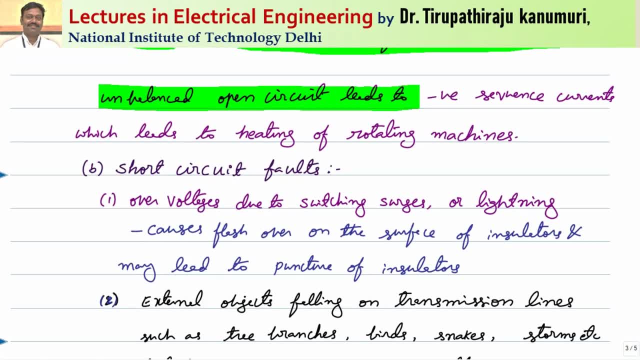 Proceeding further. so this unbalanced open circuit. so this leads to the negative sequence currents, so which leads to heating of the rotating machines. Then coming to the short circuit faults. this short circuit faults can be caused either due to over voltages, due to switching surges, or 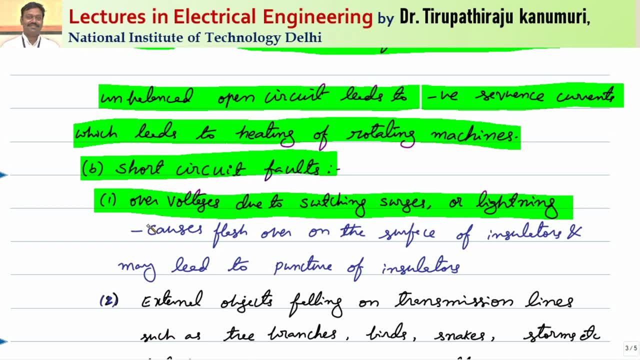 the lightning- this we already discussed in power systems in traveling waves. So what will happen during the switching transients? this gives rise to very high value of the voltages. because of this high value of voltages, this causes flash over on the surface of the insulators in the case of overhead lines, or it may lead to. 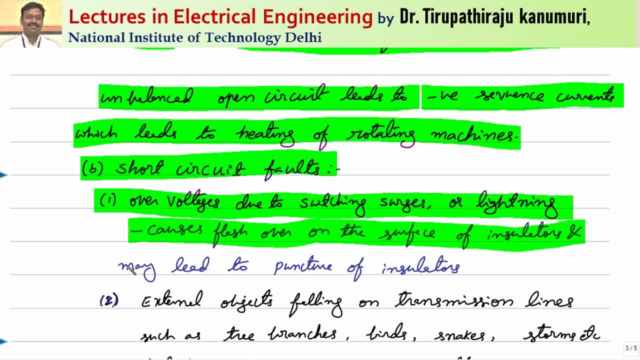 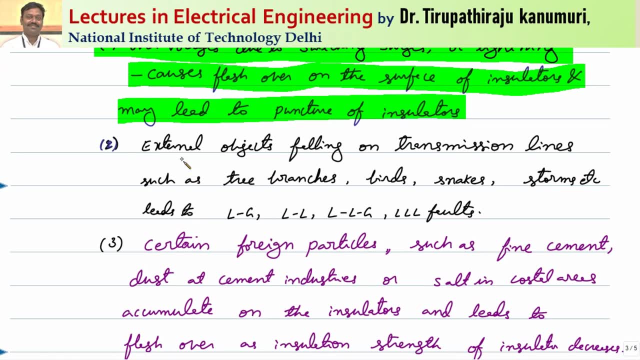 complete the dielectric breakdown in the case of cables or the machines. So this may lead to puncture of the insulators or breakdown of the insulation in the case of cables. Now coming to the second possible case. second possible reason is external objects falling on the transmission. 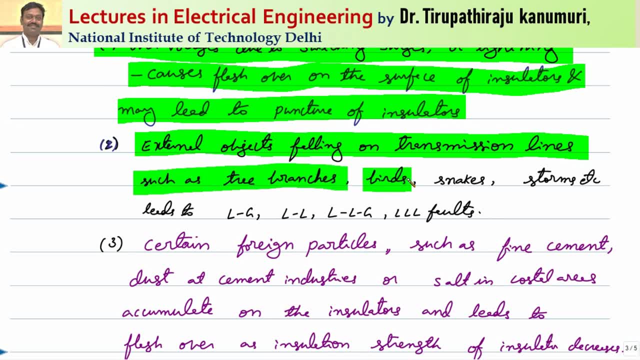 lines So, such as tree branches can fall, even birds can lead to the short circuit. sometimes the snakes also will be responsible Then. whenever the storm or the rain comes, then the conductors will move even. in that case also they may lead to line to ground fall, line to line, LLG or triple L faults. So, and one more reason that can. 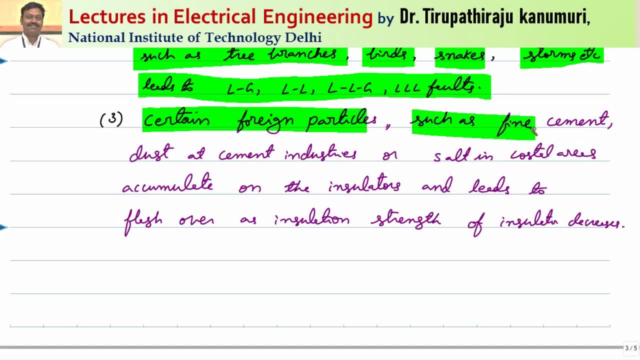 happen is certain foreign particles, such as the fine cement or dust at the cement industries or salt in the coastal areas, accumulate on the insulators and lead to flash over as the insulation strength of the insulator decreases Drastically with respect to time. So, whereas for the case of the cables, transformers or generators, 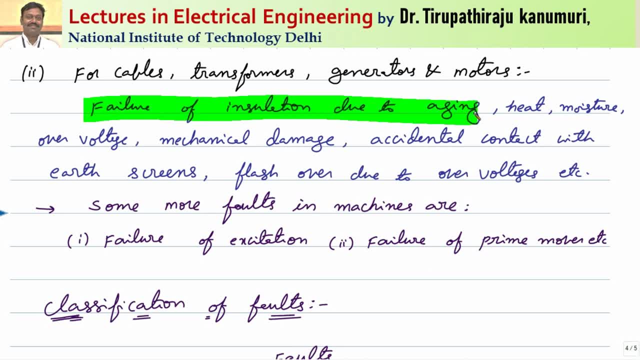 or even for the motors, the failure of insulation due to aging, heat, moisture, over voltages- this can happen during switching transients. mechanical damage, because while lying the cable or making the winding, mechanical damage can happen to the insulation. or accidental contact with the earth screens, even the flash over due to over voltages, etc. 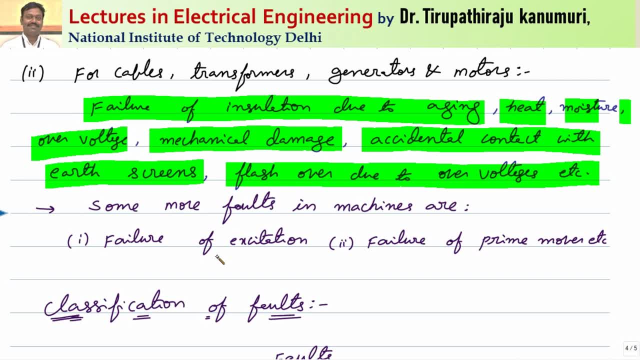 This may lead to the failure of insulation due to aging, heat, moisture, even the flash over due to the problems in the case of cables, transformers or machines. So some more problems may happen in the case of machines exclusively. they are failure of the excitation, in the case of synchronous machines, and failure of the prime over, in the case of. 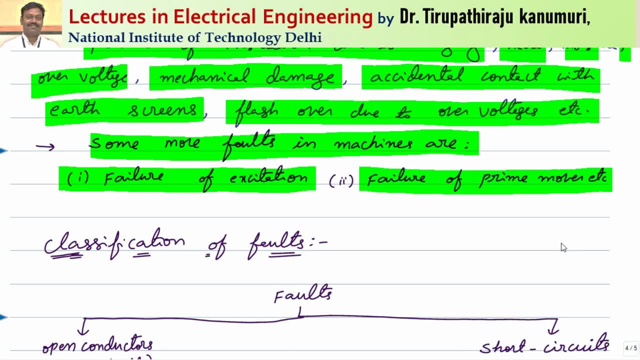 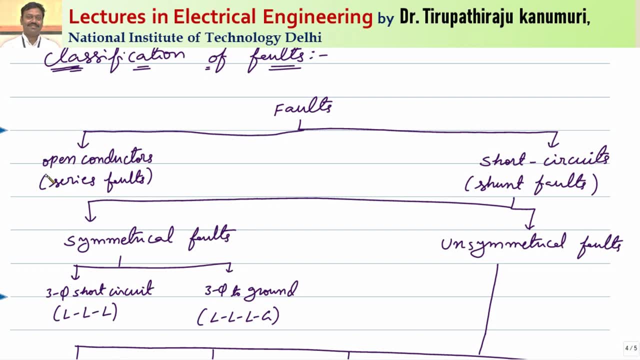 generators. These may also lead to the problem. so these things also care should be taken. So now the classification of the different faults. whatever faults we have discussed- we have already discussed this. I am summarizing here- the faults can be classified into open conductor faults or 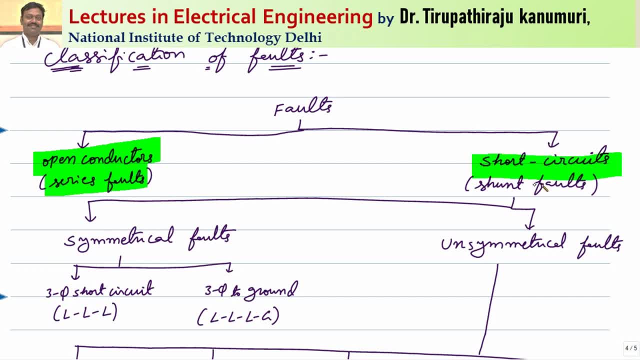 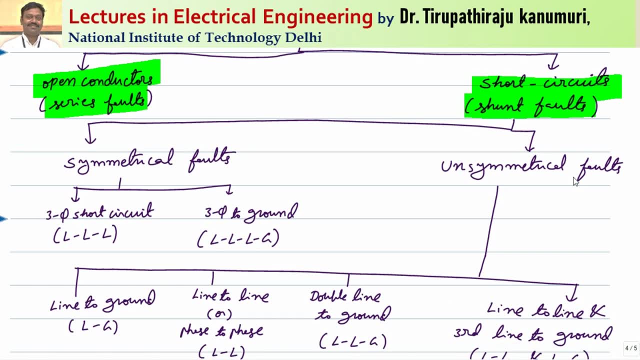 series faults and second one is short circuit or short conductor faults, or interconductor faults, or they are called as the shunt faults. So again this shunt faults or the short circuit faults, there are two types: either it is a symmetrical fault or unsymmetrical fault. Symmetrical fault: 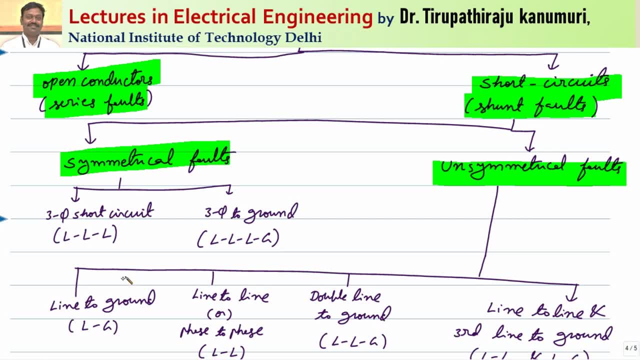 means in the all the phases the effect will be same. then it is called a symmetrical fault, then there will be no negative sequence component. then the second one can be unsymmetrical fault. in the case of unsymmetrical fault there will be a negative sequence component. 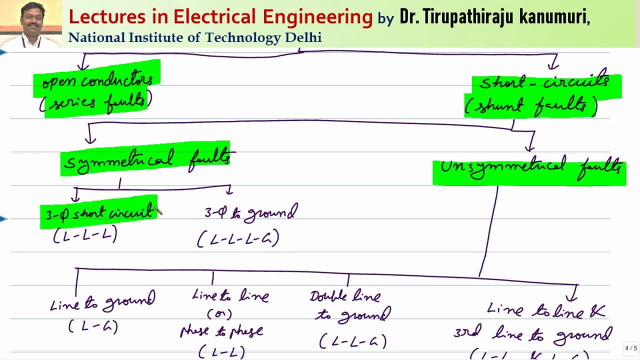 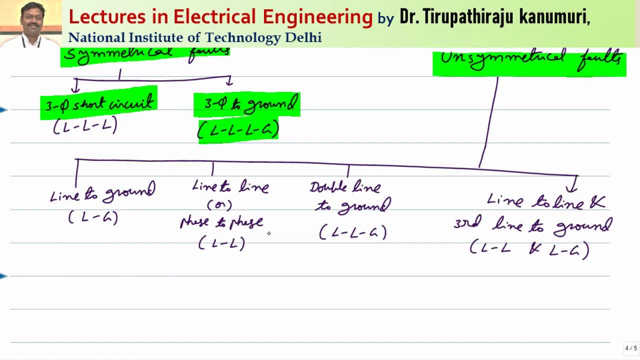 So now this symmetrical fault can be either three-phase short circuit or three-phase short circuit, along with it connected to ground. that means triple LG fault. Now coming to the unsymmetrical faults. so unsymmetrical fault: I have already discussed it can be line to ground. 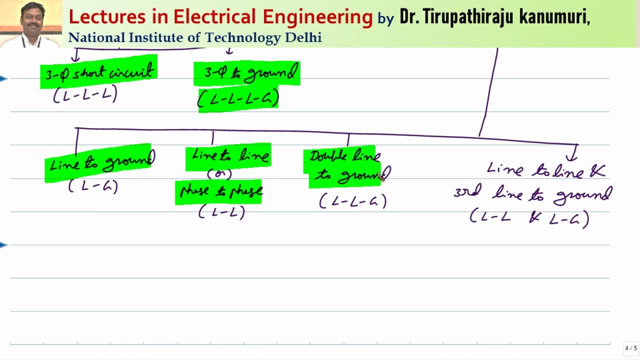 line to line, or it is also called as phase to phase fault, double line to ground fault or simultaneous faults can happen, that is, line to line fault between two conductors and this third line can be connected to ground, so it is called as LL and LG simultaneous. 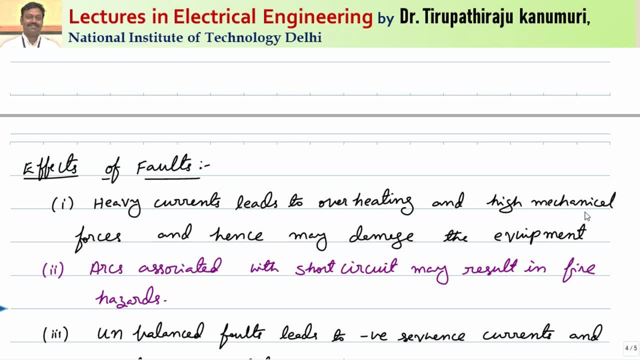 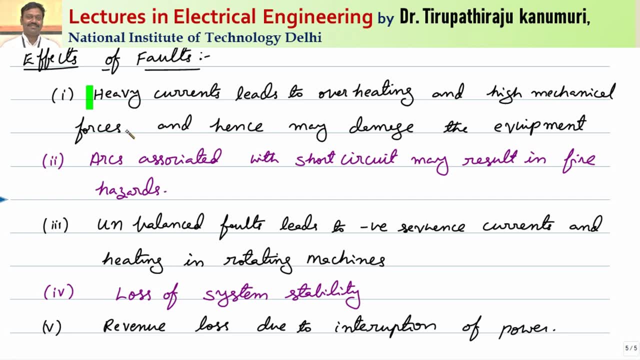 line to line and third, conductor to ground fault. So what is the effect of these faults? I am again summarizing what we have discussed. So the heavy currents will lead to overheating and high mechanical forces and hence may damage the equipment. So here, two things are there: this: 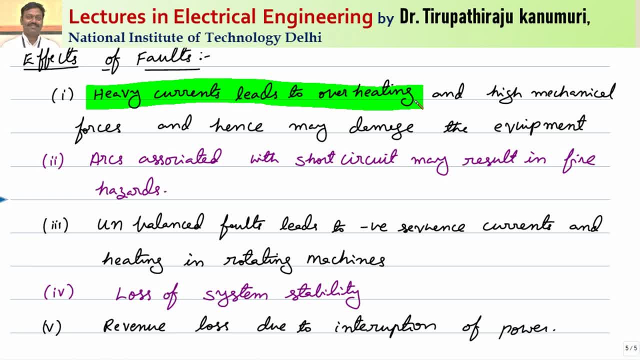 heavy currents. I have discussed it will lead to overheating. why the overheating is there? I square R. losses will be very huge. that will lead to overheating, it is known. So now second thing comes, how the mechanical forces are produced, because we know when two adjacent conductors 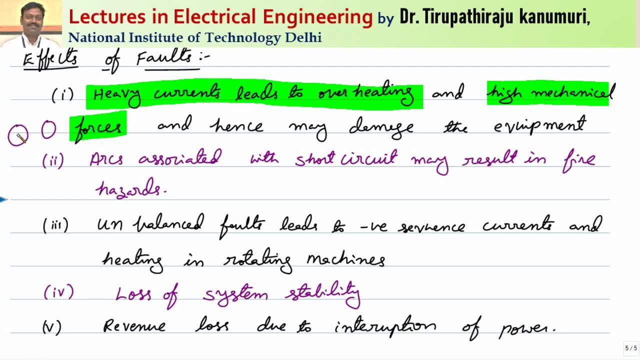 are carrying the current. so whenever the current carrying conductors are kept adjacent, whether they carry the current in the same direction or an opposite direction, a force will be experienced between them. so this force depends on what is the magnitude of the current. so if the value of 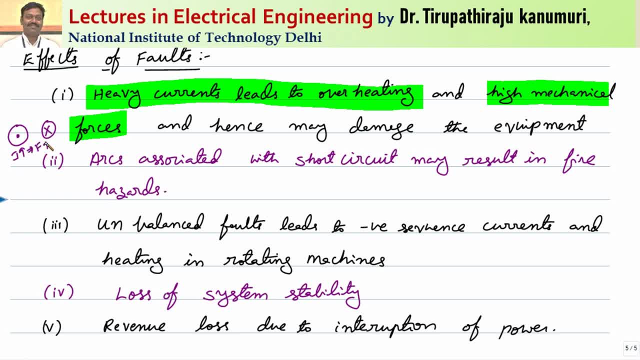 the current is increasing, so automatically the force increases. this force can be either attractive force or a repulsive force. so because of this force between the conductors, what happens? the insulation between them may get damaged, or sometimes the completely. the force is so much high that the conductor may completely come out of your complete core. that can also. 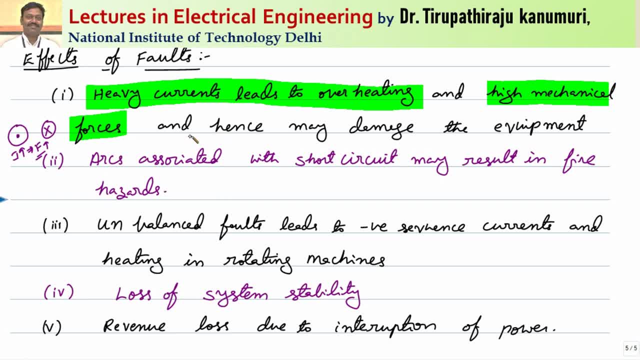 happen sometimes if the fault current is very high. this is another problem and hence may damage the equipment. So next one is the arcs associated with the short circuit may result in fire hazards. that is the second problem. because of the arcs, then unbalanced fault currents lead to negative sequence. 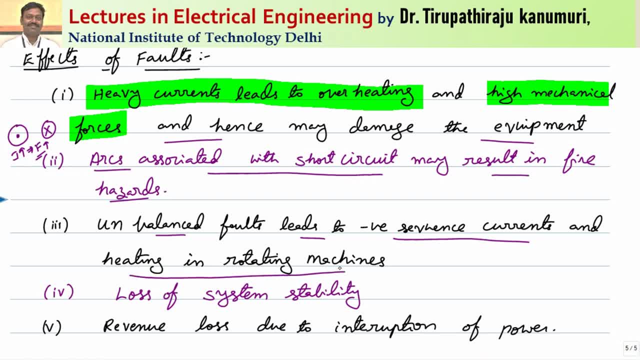 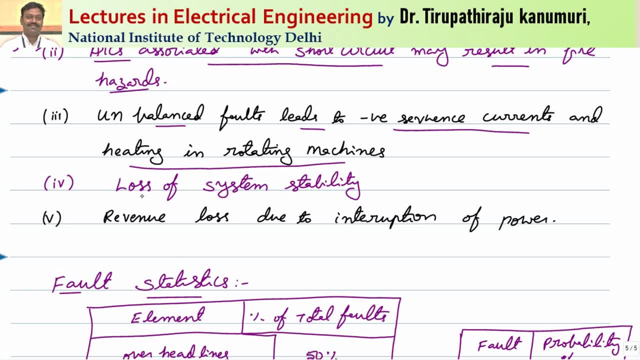 currents and hence it results in heat in the rotating machines. this is also already discussed in the case of interconnected system. if fault happens in any particular part of the power system, if the particular part is not disconnected because that fault will lead to complete instability because of mismatch in the frequencies of different alternators or different stations. 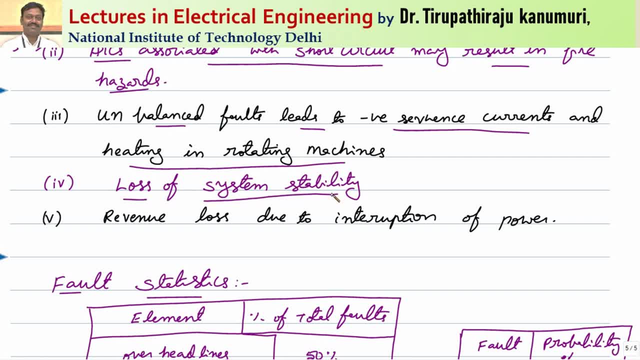 that may lead to loss of system stability. so this is the major. another problem also, and the last problem, is there will be a loss of revenue due to interruption of the fault. so because whenever the power is disconnected, there will be loss for the generating station because they don't get income, as well as there will be loss for the industries because 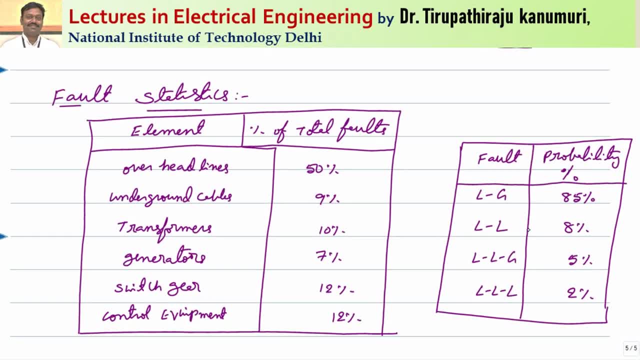 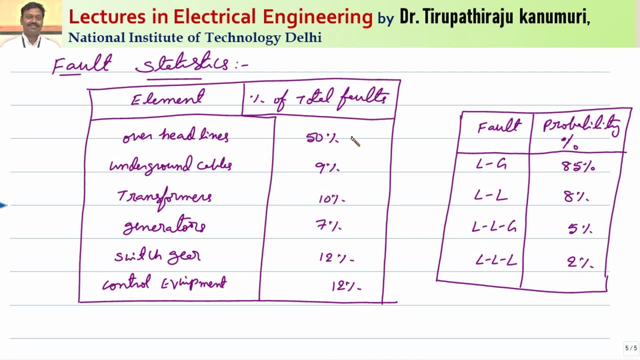 in between. if the power stop they cannot do the production, so that may lose their revenue. now coming to the fault statistics. so fault statistics: it is observed that practically overhead lines contribute for majority of percentage of the faults, because overhead line is the majority of the part in your power systems. because there is a generating station, there is a load, 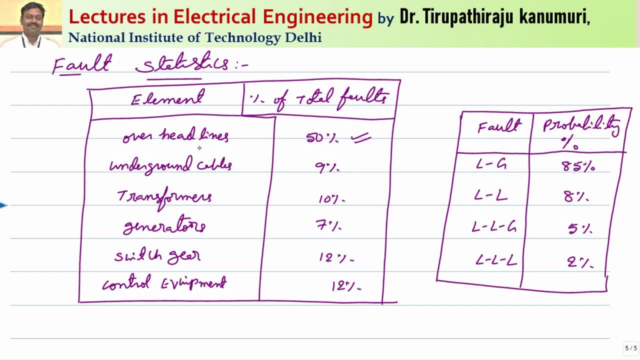 and the transmission line will be over a long distance, which will be in hundreds of meters, so obviously faults will be more in the overhead lines. and second one is it is more exposed to atmosphere so there are more chances of the faults. so in the overhead lines fifty percent. 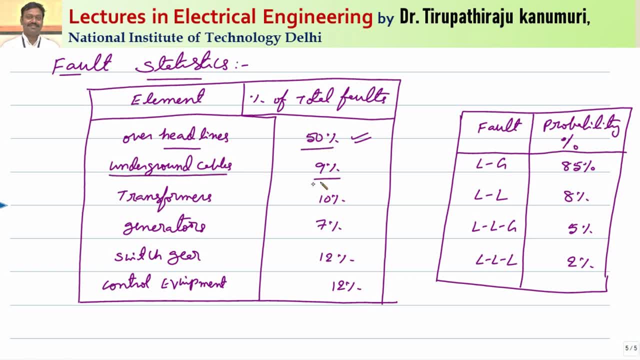 faults will happen. coming to the underground cables, there are nine percent faults. transformers: ten percent. in the case of generators or the motors, it is seven percent. in switch gear, it is twelve percent. this switch gear includes the circuit breakers, relays and all the complete parts which are responsible for protection of your system. that is called. 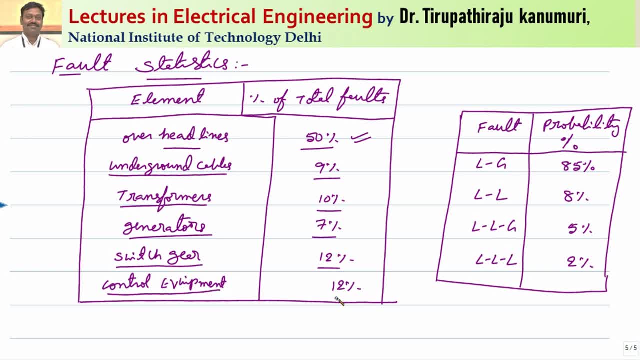 as the switch care, then that in the control equipment there is about twelve percent chances are there. so we can observe from here the overhead line is having the highest percentage. so more care should be taken for the protection of transmission lines because they contribute for majority of the faults. so now again, out of this overhead transmission line the fault happens. 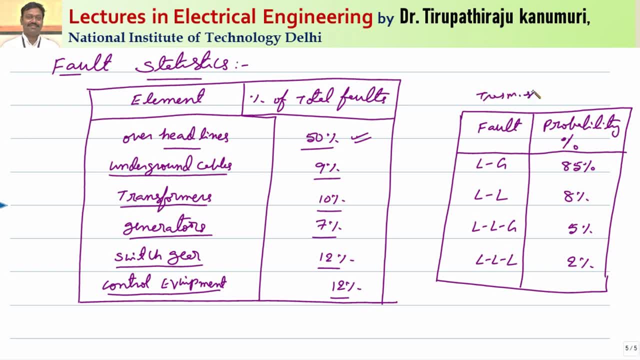 it is observed. so this is for the case of the transmission lines. please remember this. so in the case of transmission lines the line to ground faults contribute for majority of the percentage. it contributes for 85 percentage of the cases. line to line faults are eight percent, line to line to ground, or five percent and triple line. 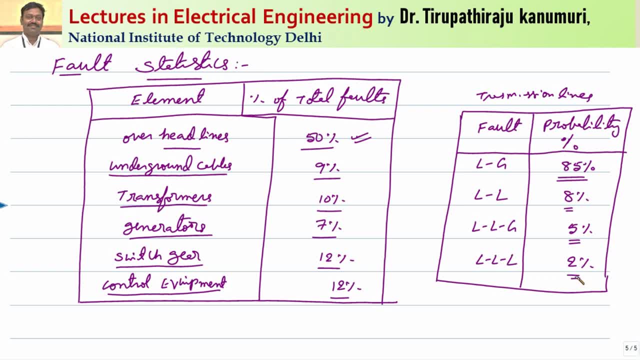 faults or balanced faults are only two percent, but out of all, the most severe are. this is the most severe type of fault, but it happens very less open and this is less severe. so but it happens most often. that's why more care should be taken for the case of lg fault and second one. most of the times this 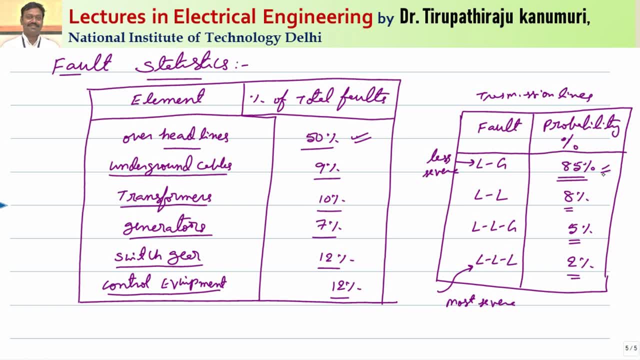 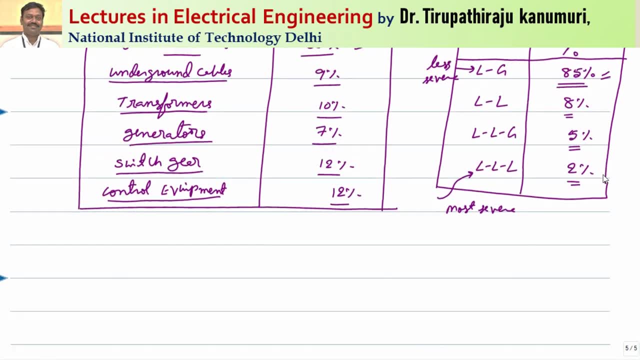 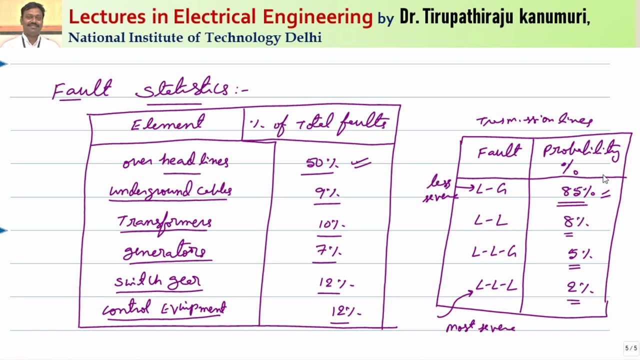 line to ground falls. they are intermittent faults. they will disconnect themselves. so that's why proper precautions should be taken while tripping your circuit for line to ground faults. so these things we are going to discuss in detail when we are discussing the protection of the transmission lines. so, finally, we can conclude from here that there is a need for protection if the 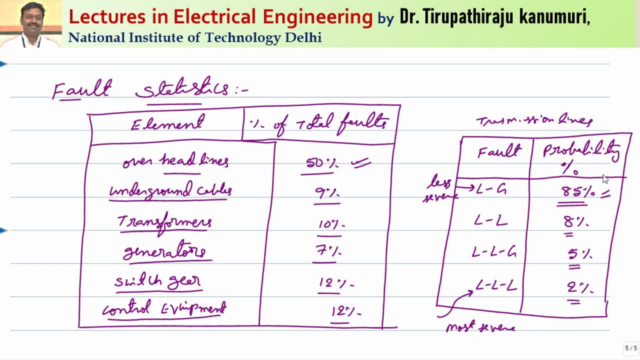 protection is not done, it may damage your equipment or it may damage your entire system and the entire system may trip. so proper precaution or the protection should be done for your transm or power system. so i hope this is clear to you in the next lecture we are